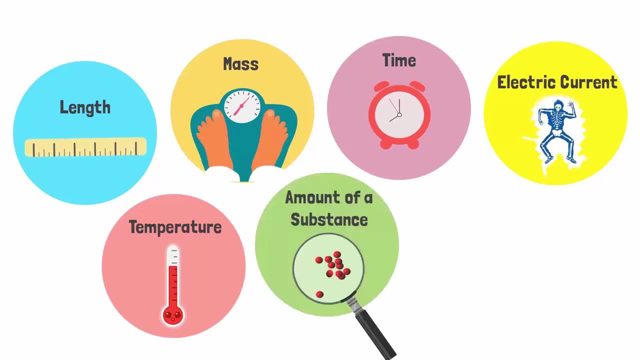 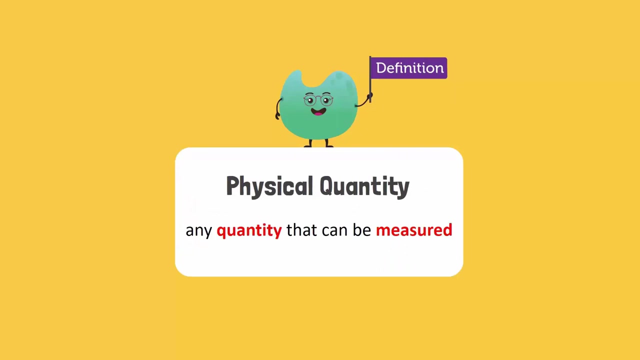 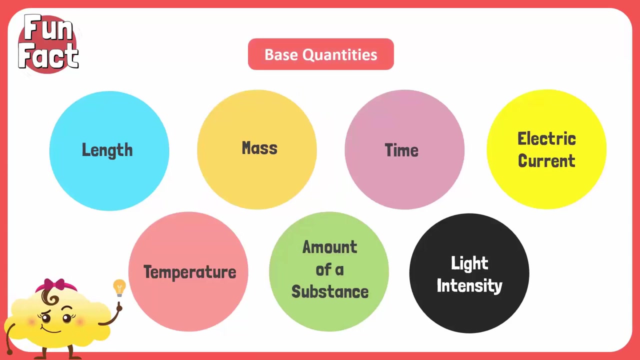 current temperature, amount of a substance, light intensity. These things are referred to as physical quantities. A physical quantity is defined as any quantity that can be measured. Did you know that these seven quantities are known as base quantities? They form the foundation or base of all other quantities. They combine to form derived quantities. For 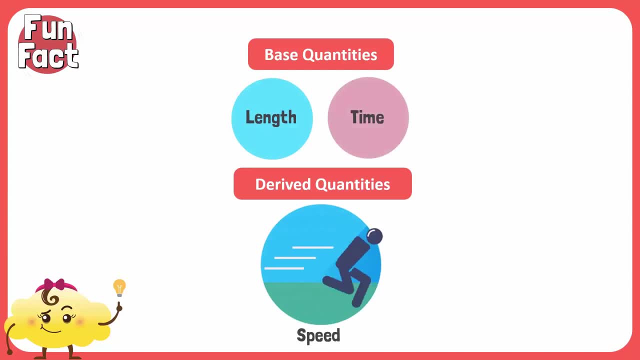 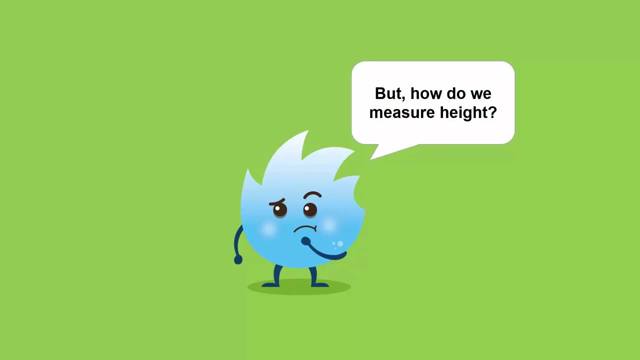 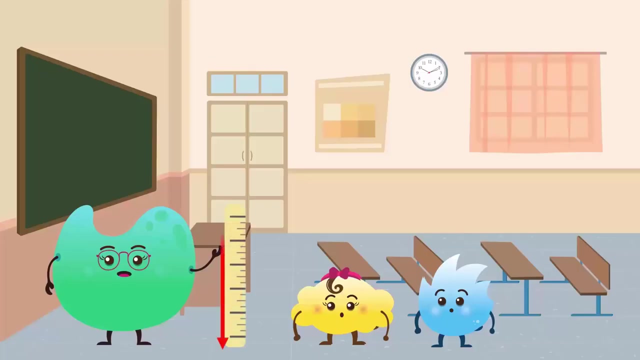 example, speed is derived from length, ie distance over time. Now that we know what physical quantities are, how do we measure them? Good question. Height is measured from the bottom to the top. To get these measurements we need units. 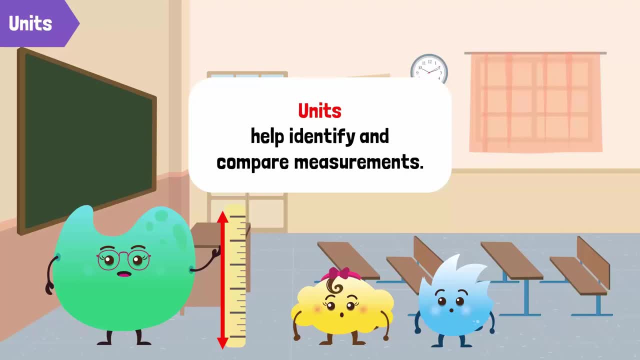 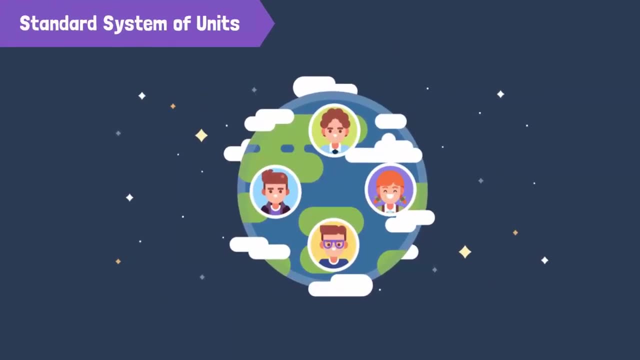 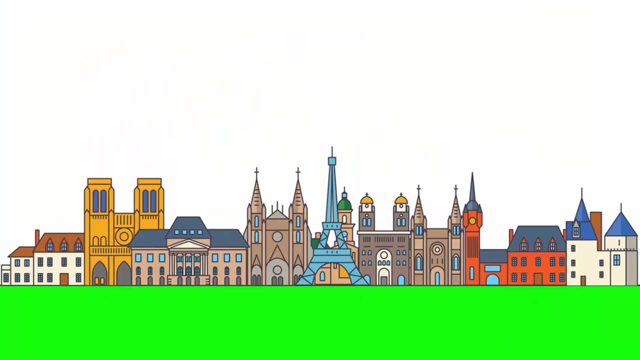 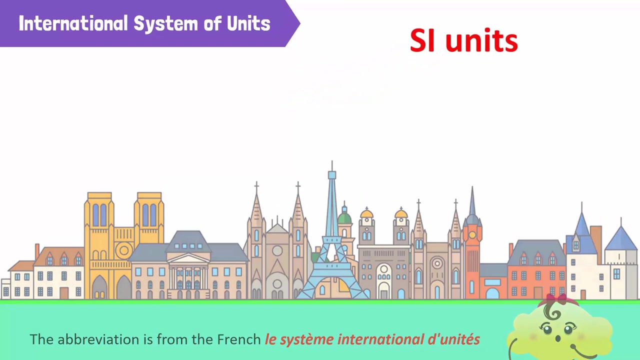 Units help us identify and compare exact measurements, For scientists and us to understand measurements around the world easily. a standard system of units was agreed upon In 1960, in Paris. such a system was created to measure the height of all the groups that managed to measure the physical quantities known as the international 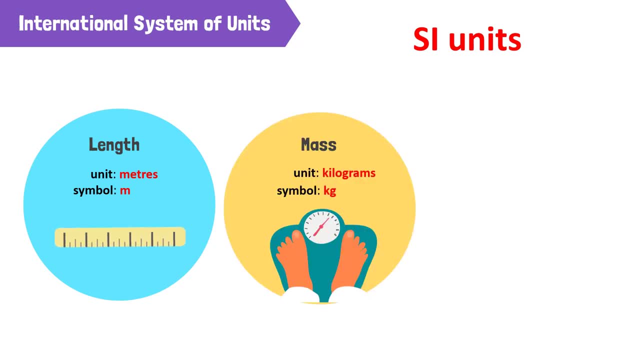 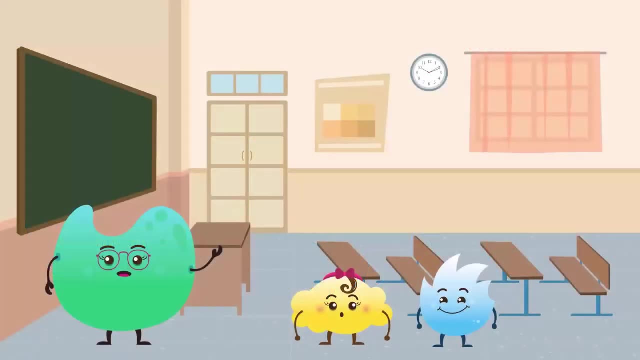 system of units- SI units for short. For example, length is measured in metres and time is measured in seconds. So to measure height we can use metres. Spiky says he is 0.5 meter tall. What does that mean? The speed of time is measured in K. 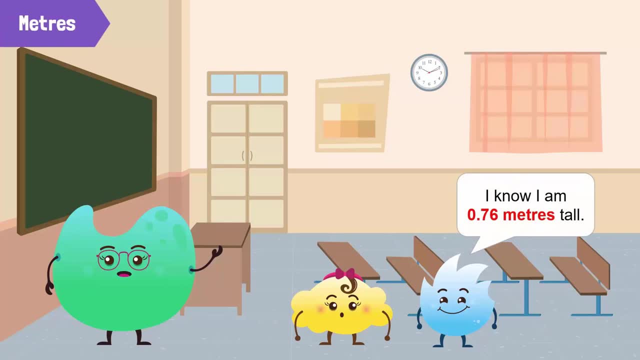 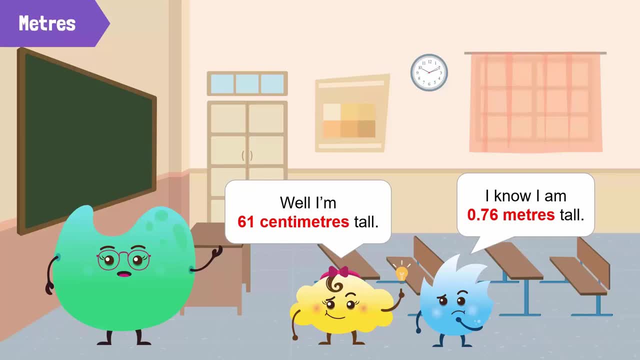 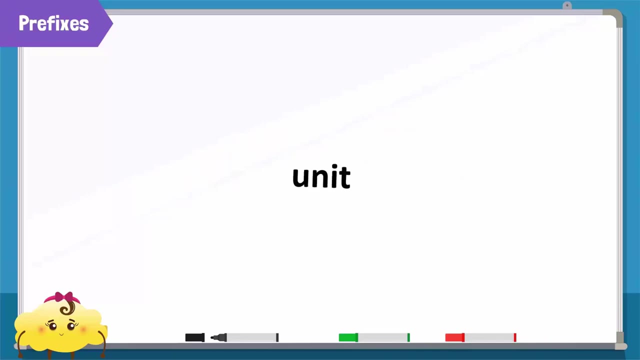 Wait, does this mean? Bubbles is taller than Spiky. What does the word centi, used before meter, mean? Let's take a closer look. Sometimes units by themselves are not enough. For instance, what if we took the mass of an ant in kilograms?